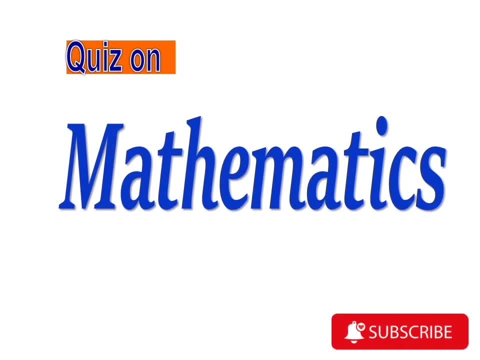 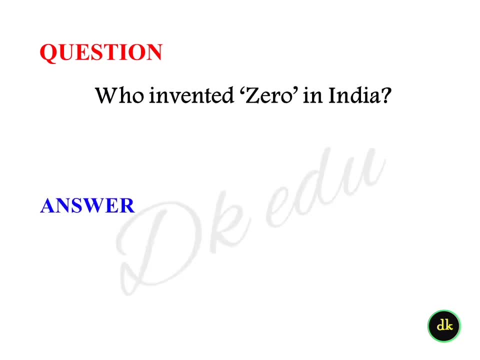 Mathematics Qs. Who invented zero in India? Answer: Arbata. Whose name was given to the first Indian satellite? Answer: Arbata. Numbers rules the universe. whose words is this? Answer: Pythagoras. When we multiply all numbers in a telephone pad, the output is Answer zero. 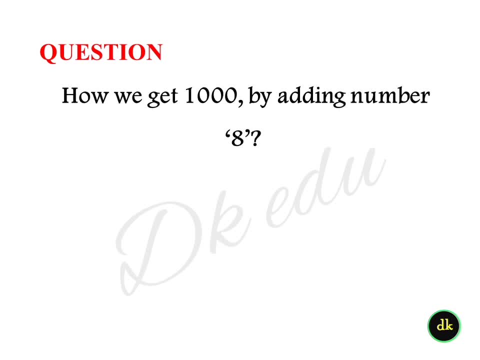 How we get thousand by adding numbers. eight. Answer: Eight hundred and eighty. eight plus eighty five, 88 plus 8 plus 8 plus 8 is equal to 1000. How many faces in a cube? Answer: 6. How many doors are there on a dice? 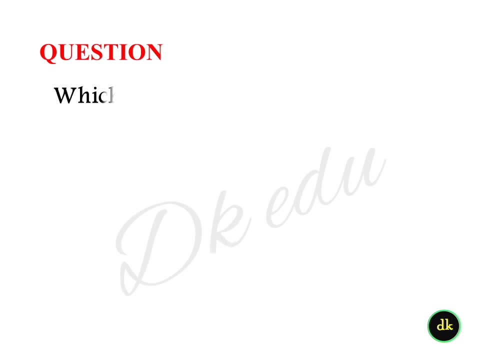 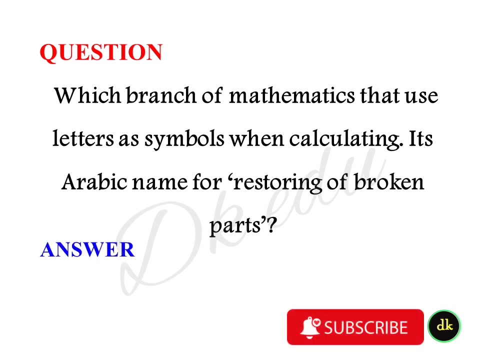 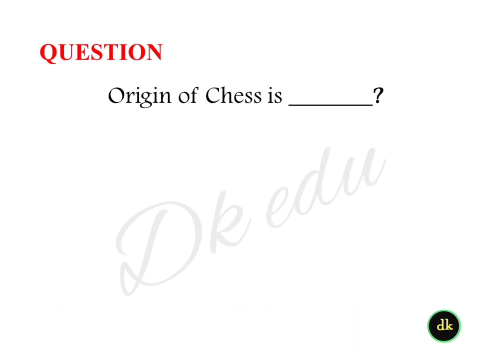 Answer 21: Which branch of mathematics that use letters as symbols when calculating Its Arabic name for restoring of broken parts? Answer: Algebra: Origin of chess is dash. Answer: India. Complete the series 52,, 59, 66. Answer 73, 83, 80 and 87. The number 50 is the 25% of a number. 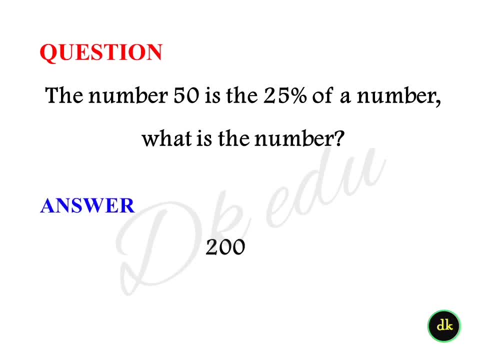 What is the number? Answer 200, Which comes after million dash. Answer: Trillion 625 is divided by 25 is equal to 100.. How many faces in a cube? Answer 2. How many faces in a cube? Answer 1: How many faces in a cube. 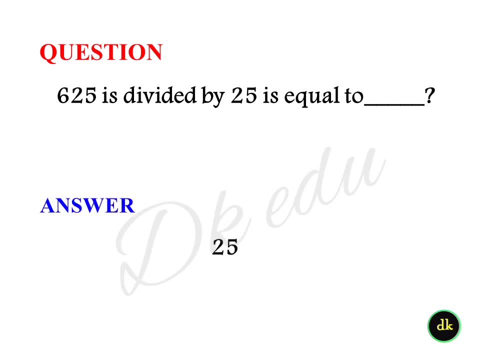 Answer 2: How many faces in a cube. Answer 2: How many faces in a cube. Answer 3: How many faces in a cube. Answer 4: How many faces in a cube. Answer 5: How many faces in a cube. Answer 6: How many faces in a cube. 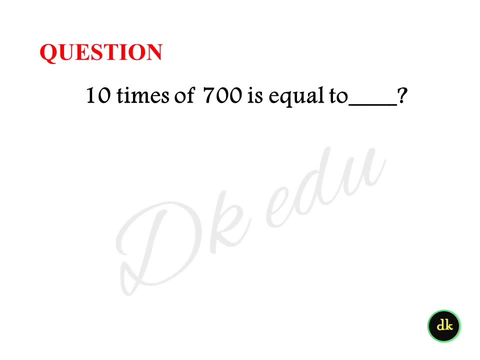 Answer 6: How many faces in a cube. Answer 7: How many faces in a cube. Answer 8: How many faces in a cube. Answer 9: How many faces in a cube. Answer 10: How many faces in a cube. Answer 10: How many faces in a cube. 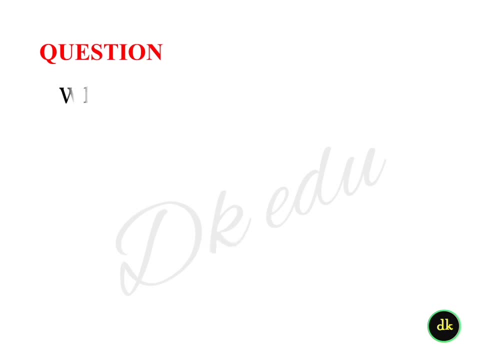 Answer 11: How many faces in a cube. Answer 12: How many faces in a cube? Answer 13: How many faces in a cube. Answer 14: How many faces in a cube. Answer 15: How many faces in a cube. Answer 16: How many faces in a cube. 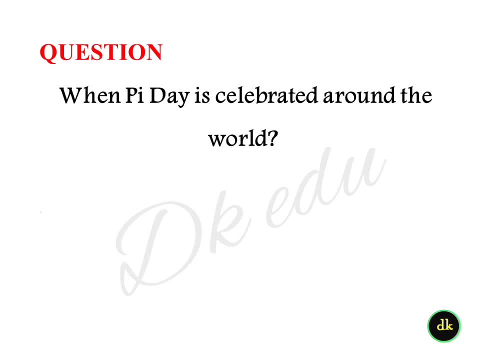 Answer 17: How many faces in a cube? Answer 18: How many faces in a cube? Answer 19: How many faces in a cube? Answer 20: How many faces in a cube. Answer 21: How many faces in a cube? Answer 22: How many faces in a cube. 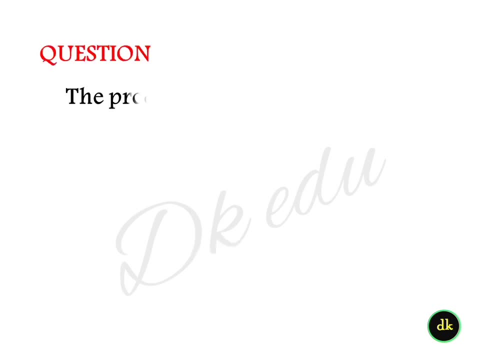 Answer 23: How many faces in a cube? Answer 24: How many faces in a cube? Answer 24: How many faces in a cube. Answer 25: How many faces in a cube. Answer 26: How many faces in a cube. Answer 27: How many faces in a cube. 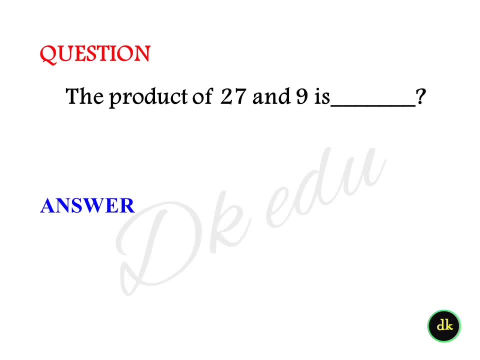 Answer 28: How many faces in a cube? Answer 29: How many faces in a cube? Answer 30: How many faces in a cube? Answer 31: How many faces in a cube? Answer 32: How many faces in a cube? Answer 32: How many faces in a cube. 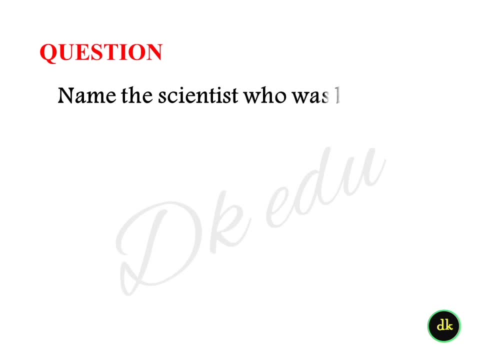 Answer 33: How many faces in a cube? Answer 34: How many faces in a cube? Answer 35: How many faces in a cube? Answer 36: How many faces in a cube? Answer 37: How many faces in a cube? Answer 38: How many faces in a cube. 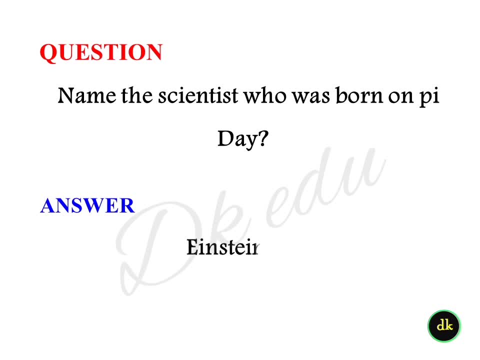 Answer 39: How many faces in a cube? Answer 40: How many faces in a cube? Answer 41: How many faces in a cube? Answer 42: How many faces in a cube. Answer 43: How many faces in a cube? Answer 44: How many faces in a cube. 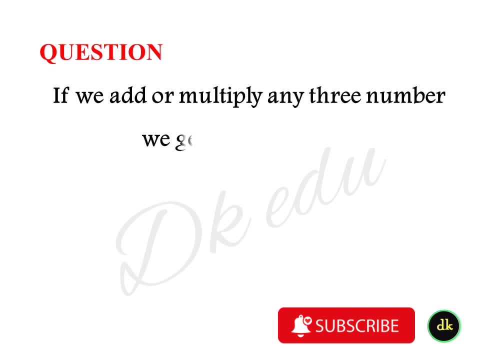 Answer 45: How many faces in a cube? Answer 46: How many faces in a cube? Answer 47: How many faces in a cube? Answer 48: How many faces in a cube. Answer 49: How many faces in a cube? Answer 50: How many faces in a cube? 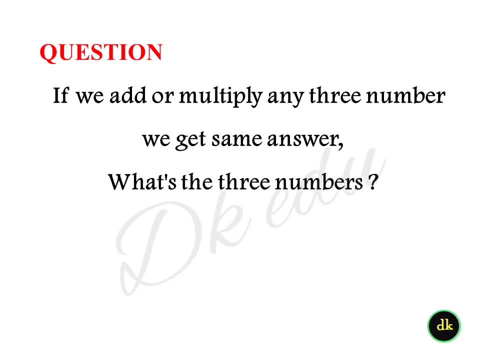 Answer 51: How many faces in a cube? Answer 52: How many faces in a cube? Answer 53: How many faces in a cube? Answer 52: How many faces in a cube? Answer 53: How many faces in a cube? Answer 54: How many faces in a cube. 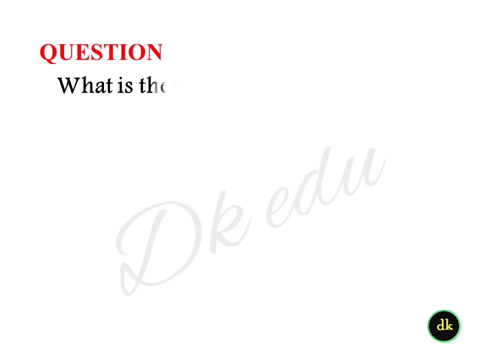 Answer 55. How many faces in a cube? Answer 56: How many faces in a cube? Answer 57. What is the value of x in the equation 7-x equal to Answer 47. What is the formula to calculate the area of a semicircle? 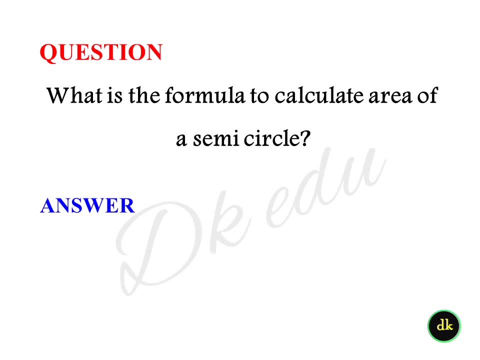 Answer 58: How many faces in a cube? Answer 59: How many faces in a cube? Answer 60: How many faces in a cube? Answer 71: How many faces in a cube? Answer 6,, 8,, 10.. A triangle is a two-dimensional or three-dimensional in shape. A two-dimensional shape. 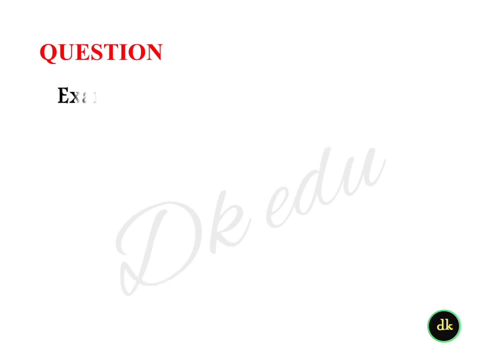 Example of two-dimensional shapes: Answer: Triangle: circle, semi-circle, square and rectangle. All the sides of the dash triangle are equal. Answer: Equilateral- The largest and smallest Four-digit number: Answer: Largest is 9,999 and smallest is 1,000.. 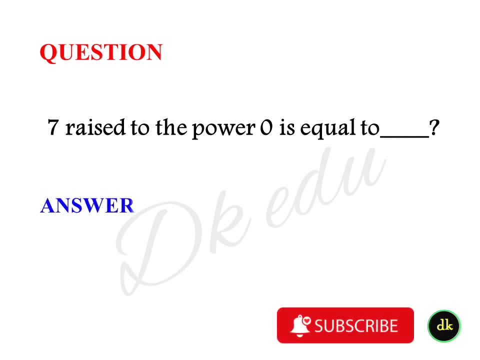 7, raised to the power 0, is equal to Answer 1.. The cube of 9 is Answer 729.. The value of pi. The value of pi is equal to Answer 3.14.. What is the cube root of 3,375? Answer 15.. 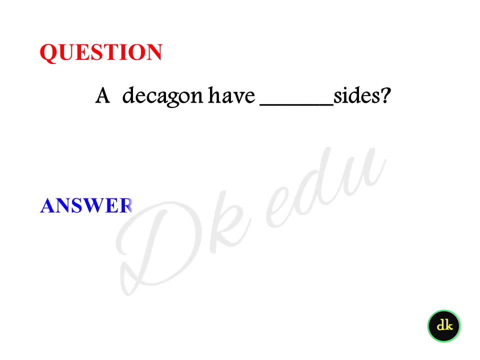 A decagon has dash sides. Answer 10 sides. How to calculate the area of a rectangle? Answer Length into breadth. Who was the first to use the Greek letter pi to denote the constant Answer: William Jones. What is the value of a raised to 0?? 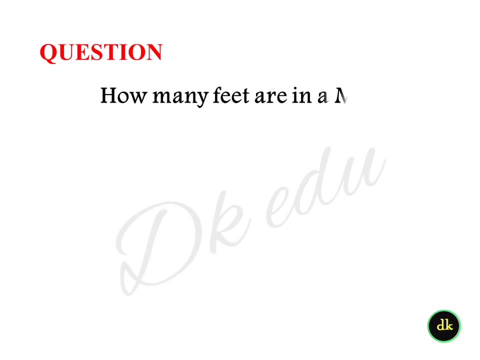 Answer 1.. How many feet are in a mile? Answer: 5,280.. Answer: 5,280.. We know that the petals of flowers follow a number series. Do you know what it is? Answer: The Fibonacci series. 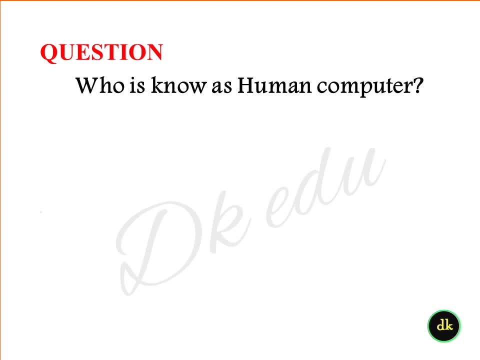 Who is known as human computer? Answer: Shangudala Devi. Apple sog-i long. The longest side of theabeth's'vecube' is 5,280.. Answer: 5,280.. side of a right-angled triangle is called as Answer hypotenuse. Who is the best mathematician?